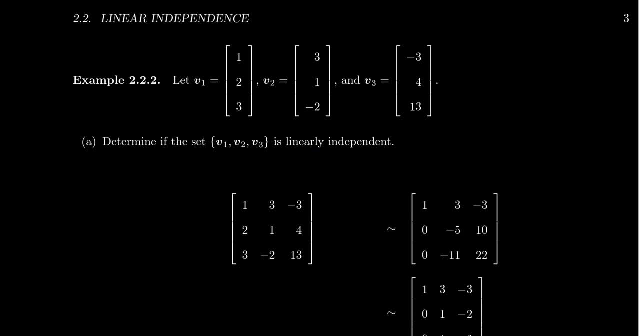 independent. Remember, linearly independent means we're looking for. well, we're trying to consider the following problem: Can we find coefficients C1, C2, and C3 so that, given those choice of vector, of those choice of scalars, C1, C2, C3, can we combine the vectors to give you 0? Now, 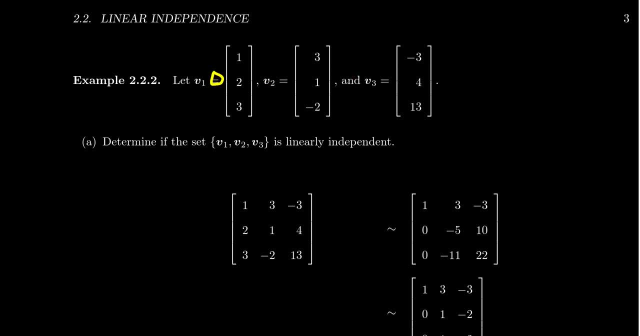 there's always one way of doing that right. We can always just slap in the scalars 0,, 0,, 0. That'll give us the 0 vector. But that's a trivial way of doing that. Can we have a non-trivial way? 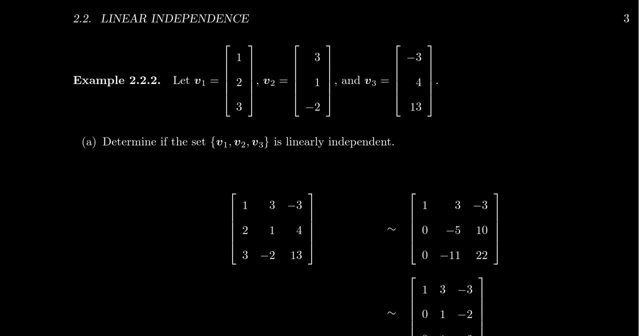 of producing the 0 vector. If you can't do that, we say the vectors are linearly independent. If there is some non-trivial way of doing it, we say the vectors are linearly dependent. Now suppose we form a vector. 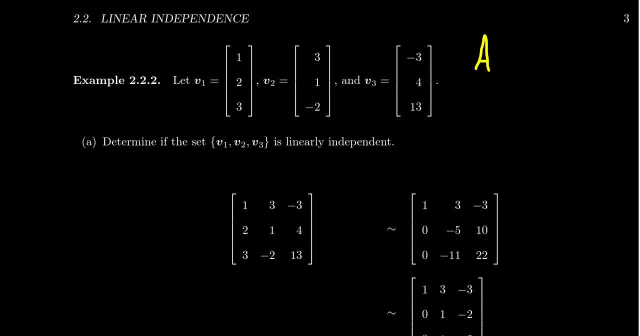 Well, a matrix A whose column vectors are exactly just the Vs, V1,, V2,, V3, right here. So trying to find a combination that equals 0 says we're trying to look for a vector X, so that A times X is equal to the 0 vector. This matrix equation represents a homogeneous system. 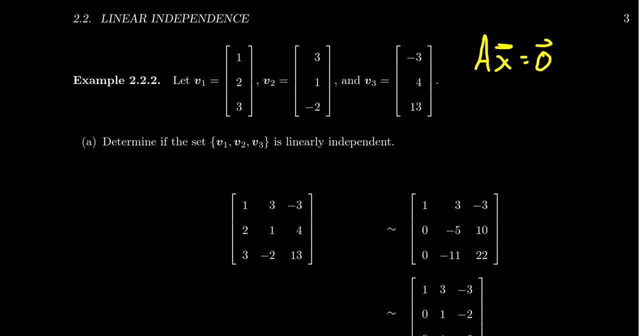 of equations And we're trying to figure out: are there solutions to this homogeneous system? We don't really care about whether it's consistent or not, because we know it's consistent. We have, for example, the non or the trivial solution. X equals 0.. We're trying to figure out: are there non-trivial? 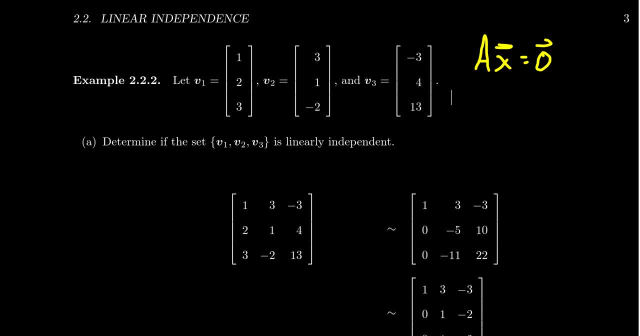 solutions, which would come down to finding out: is this linear system, does it have multiple solutions or not? At the beginning of this course, we call that the dependent case, And this is actually why we call it that: that the dependent case, that is, there's multiple solutions to AX. 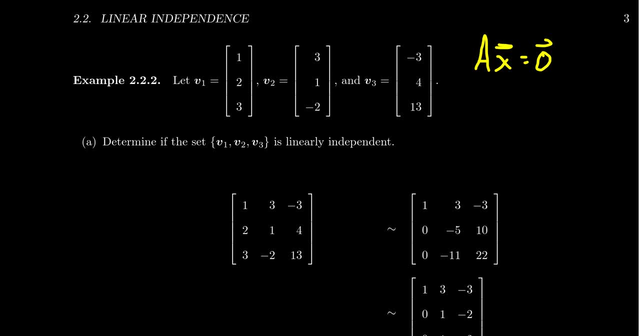 equals 0, is because the column vectors in play are linearly dependent. So we're trying to ask ourselves: are there, are there non-trivial solutions to this system of equations here? Now, in order to work with that, we of course we're going to set up a augmented matrix where the coefficient matrix that you see. 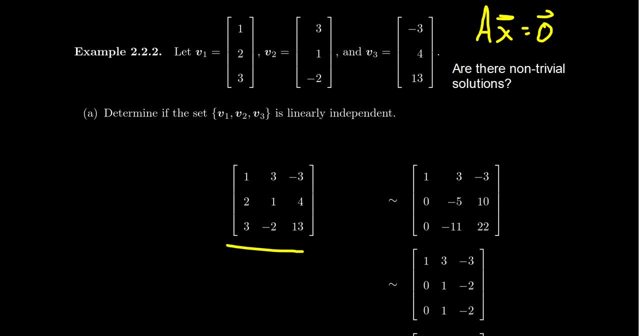 right here is just going to be the like. it's just the matrix A from above. Its first column is V1, its second column is V2, its third column is V3.. Now, to be proper, we should be augmenting this. 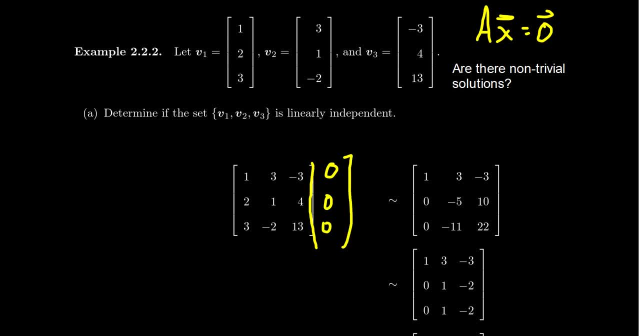 with the zero vector 0,, 0,, 0.. You'll notice that I originally omitted that. Why would I do that? We'll actually see in a moment why that is So if we're trying to solve this system of equations. 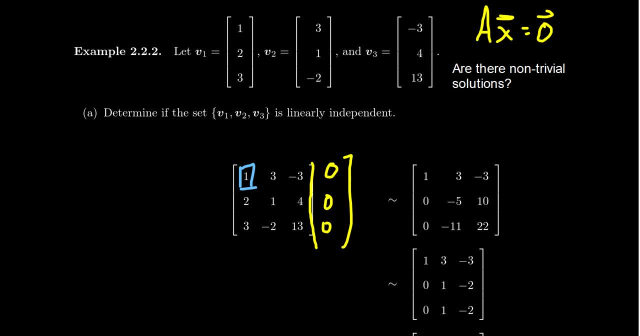 we look at the 1, 1 position. There's already a 1 there, which is great. To get rid of the 2 below it, we're going to take row 2 minus 2 times row 1.. And to get rid of the 3 below, we're going to 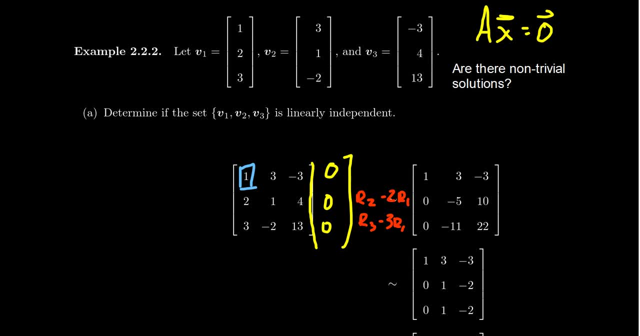 take row 3 and minus 3 times row 1.. So we're going to get minus 2,, minus 6,, plus 6, and minus 0.. We're going to get minus 3,, minus 9,, plus 9, and then minus 0.. Notice that 2 minus 2 is 0.. 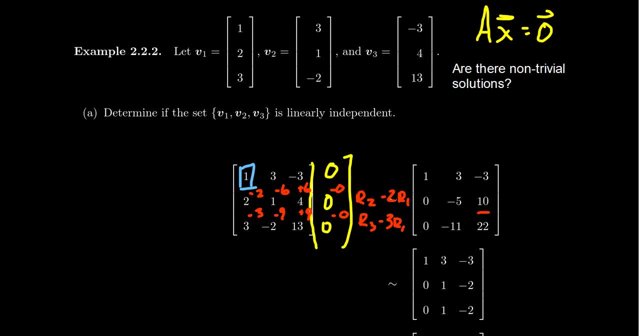 1 minus 6 is negative 5.. 4 plus 6 is 10.. And then the next one: you're going to get 0 minus 0,, which is still 0.. All right, Here you're going to get 3 minus 3, which is 0.. Negative: 2 minus 9. 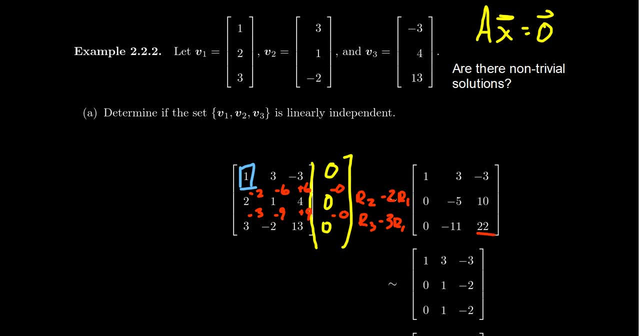 is a negative 11.. 13 plus 9 is 22.. And then you're going to get 0 minus 0 again, which is just 0.. And so, notice, had we kept the column at the end, which is 0, 0, 0,, it didn't change when we did these row operations. All right. 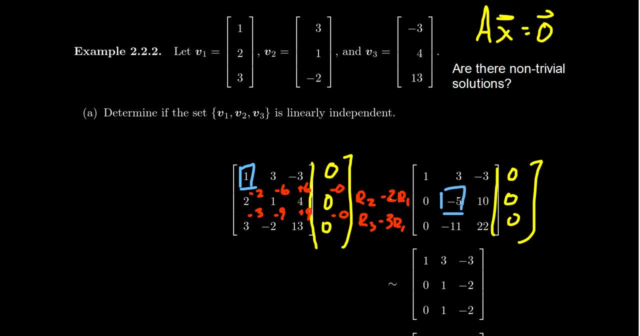 Well, moving on to the next pivot position, notice that in the second row, everything's divisible by 5.. We have a negative 5,, a 10, and a 0, right, If we were to divide everything by negative 5,. 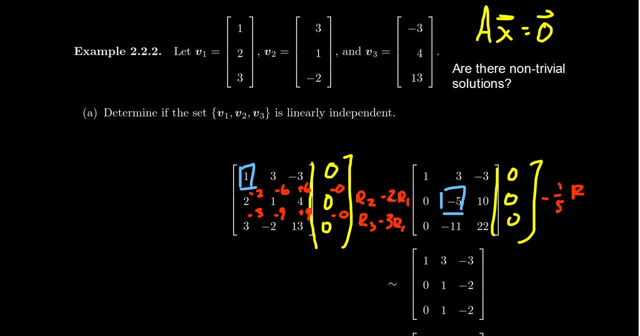 so I get a 1 in that spot, you get a negative 1. fifth row 2.. Oh, since I'm added, looking at the third row, everything's divisible by 11. right there, I'm going to divide by negative 11 for. 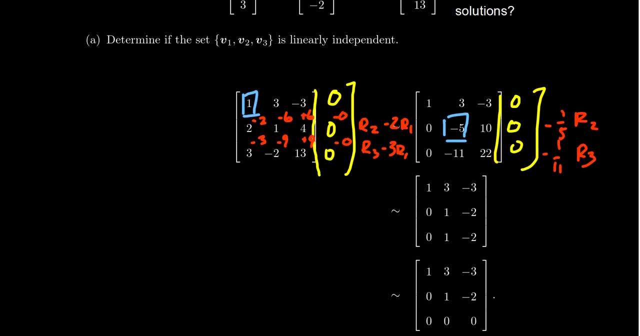 3.. And so what then happens is that negative 5 becomes a 1,, 10 becomes a negative 2.. But what happens to the 0?? 0 divided by negative 5 is still a 0. And negative 11 divided by negative 11 is a. 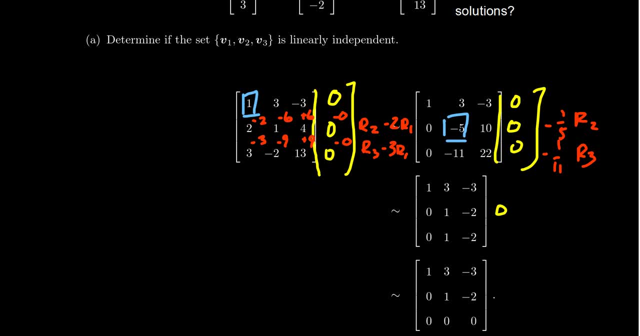 1, right: 22 divided by negative 11 is a negative 2.. And then 0 divided by negative 11 is still a 0. We didn't do anything in the first position, So notice, when we did row replacements, the 0s. 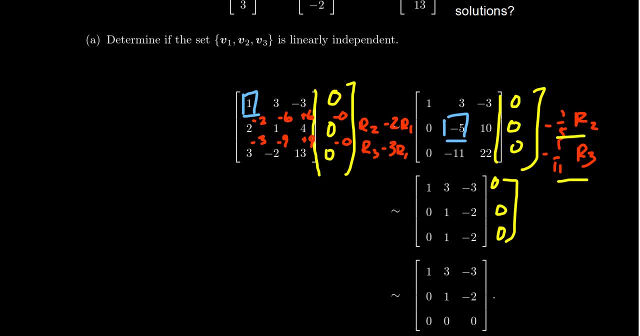 don't change When you do scaling, the 0s in that last column don't change. For some reason we had to do the interchange operation, maybe because we wanted to switch the rows. You're just going to swap a 0 with a 0, and the 0s don't change. So one thing to observe. 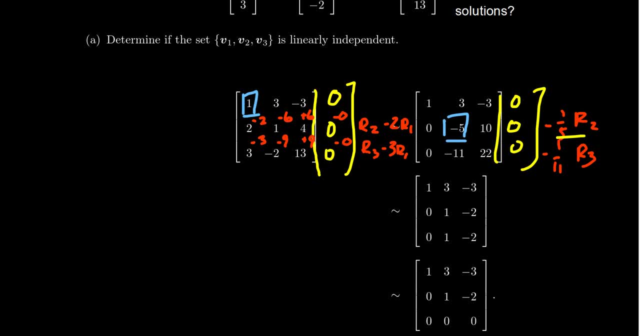 here is that when you're working with a homogeneous system of equations, the three row operations will never change a column of 0s to be anything other than a column of 0s And as such, we often just omit that augmented column for these homogeneous systems here, because I know nothing's going to. 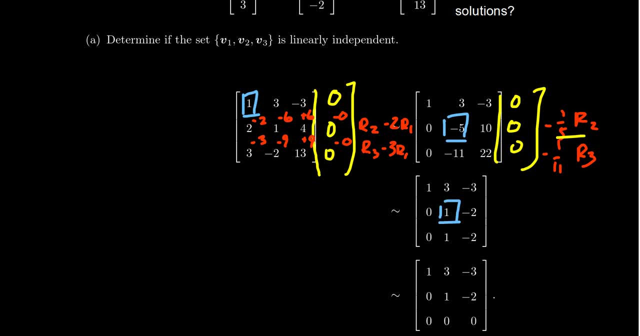 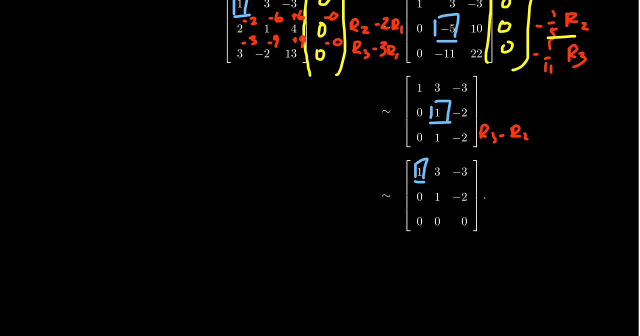 happen because arithmetic-wise it's not offering us anything. To get rid of the 1 below our current pivot position, we're going to take row 3 minus row 2. And that thus gives us the matrix that you see. right here We have a pivot. We had a pivot column in the first one and the second one We now 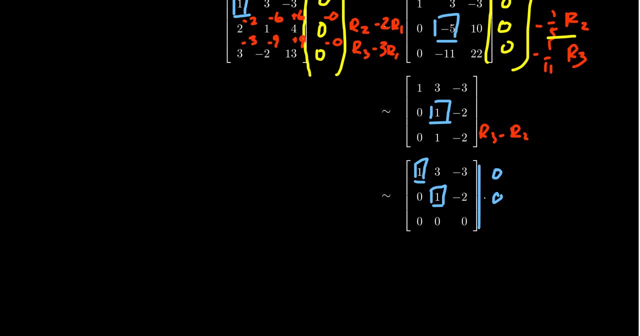 get this row of 0s right, which, if we throw in that augmented column here, this last one, just says that 0 equals 0. There's no problem with that. This system is consistent. There is no issue about consistency. But one thing I should mention here is that, because of this last column, 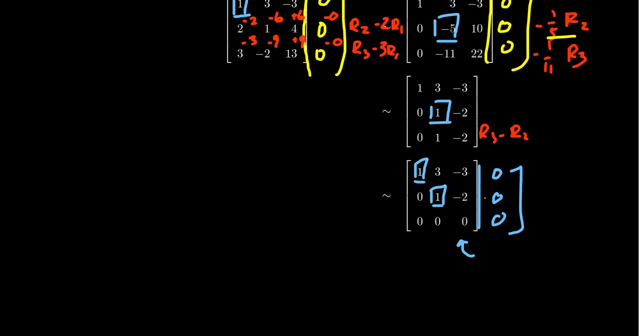 lacking a pivot. here we do see that this non-pivot column produces a free variable, And what we've seen in the past is that a consistent system has multiple solutions exactly when it has a free variable. So what we see here is that this system does, in fact, have multiple solutions. These multiple 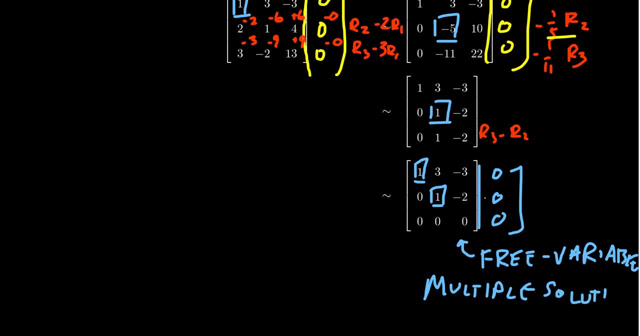 solutions are not consistent. They're not consistent, They're not consistent, They're not consistent Other than the zero vector itself. these multiple solutions are going to give us non-trivial solutions to the homogeneous system. Non-trivial solutions. And since we have non-trivial solutions, this tells us that the set 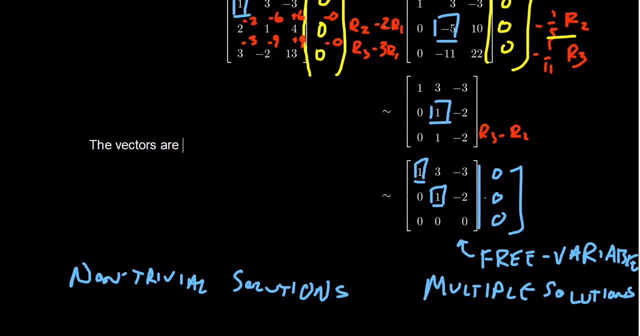 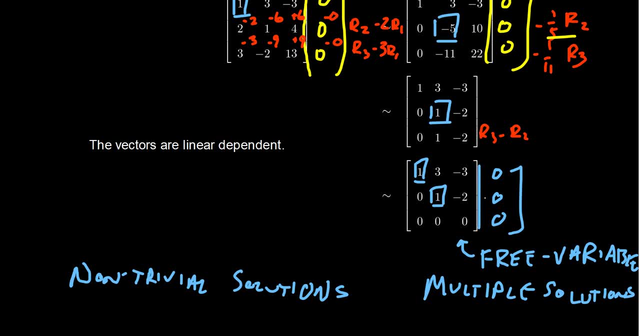 of vectors. So basically, when you have a set of vectors, we can write them as the columns of a matrix. You row reduce that matrix. If you row reduce that matrix and you have any non-pivot columns, then that means the set of vectors were linearly dependent If every column turned out to. 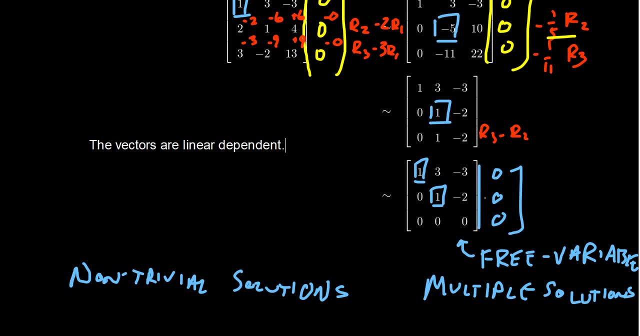 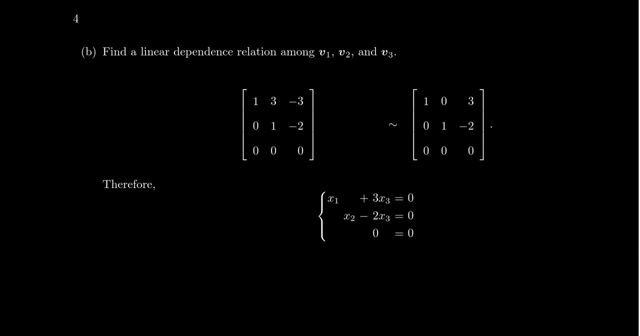 be a pivot column. that would mean the vectors are linearly independent, And we'll see an example of that one sometime in the next video here. Now, since we have a set of vectors which are literally, it then is relevant to start looking for a linear dependence relationship. can we find? 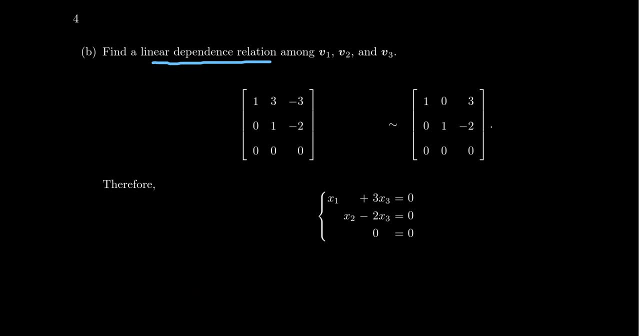 non-zero coefficients that when combined together with the vectors, we can produce the zero vector. well, we're going to continue to row reduce our matrix right here. so this matrix was an echelon form, but it's not on row reduce echelon form to get a row reduced, we're going to take row one. 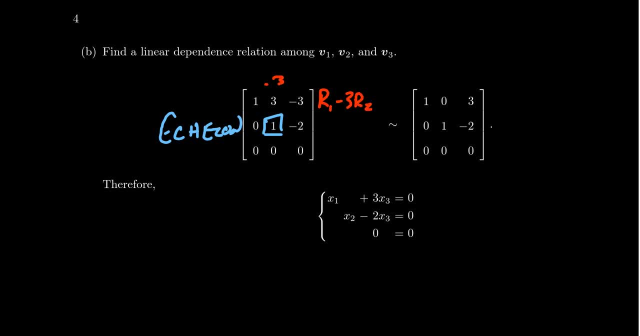 minus three times row two. so we get minus three right here and we're going to get plus six right here, and so this matrix, right here is our rref row reduced echelon form. if we were to translate it back, uh well, if you take this system right here, we could do this one right here. no, not a big deal. 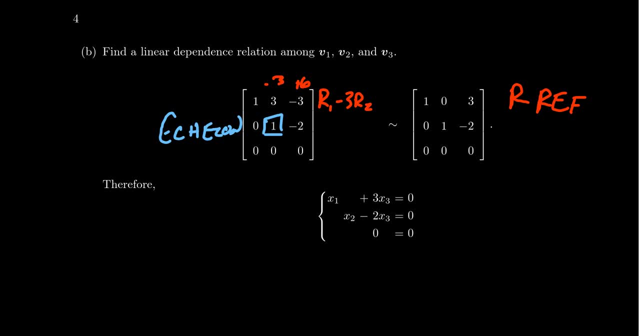 i'm sorry. uh, we wanted to be doing this one right here. this is, this is the one we're doing. so if we translate the rref back into a system of linear equations, you'll see that that x1, right plus 3x3 is equal to zero. I'm omitting in this example. I was omitting that. 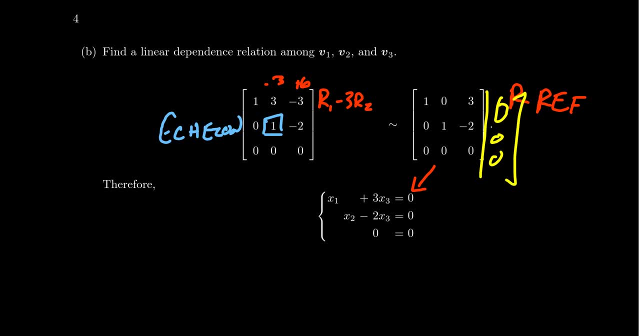 augmented column, because it's just the zero column, which never changed when we do these row operations. But realizing this is a homogeneous system of equations, we should have a column of zeros right here. So we see that 1, 0, 3 means to us 1x1 plus 0x2 plus 3x3 equals zero. And then we 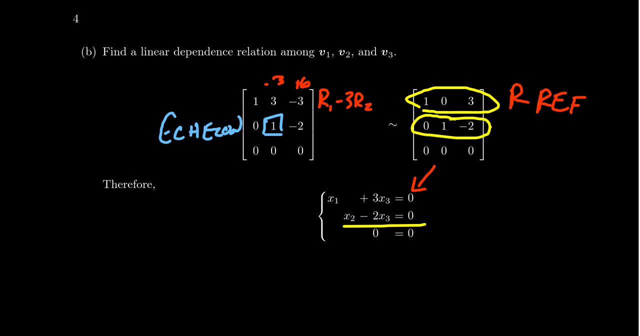 also for the next row, the 0, 1, negative 2,. this tells us that 0x1 plus 1x2 minus 2x3 equals zero. And then the last column, the last row of zeros, is just the equation 0, 0,, which really means that. 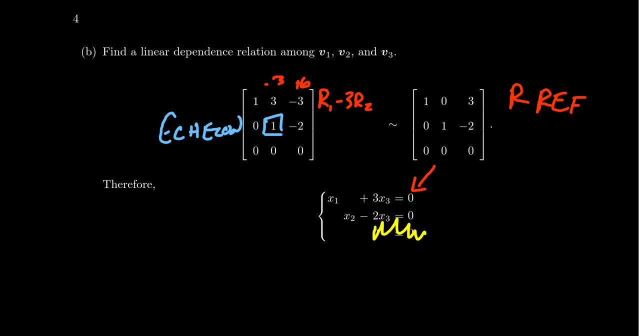 we do not need it whatsoever. Now, taking the two equations we have in hand- because there was no pivot in the third column, that's our free variable- Solve for the dependent variables with respect to the free variables, And when we do that we'll end up with x1 is equal to negative. 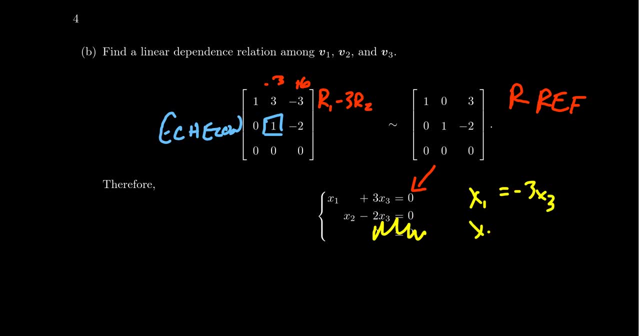 3x3 and x2 is equal to negative- sorry, positive- 2x3.. This is a free variable, And so we could then set x3 to be whatever we want. If we set x3 to be zero, then x1 and x2 would likewise be zero. 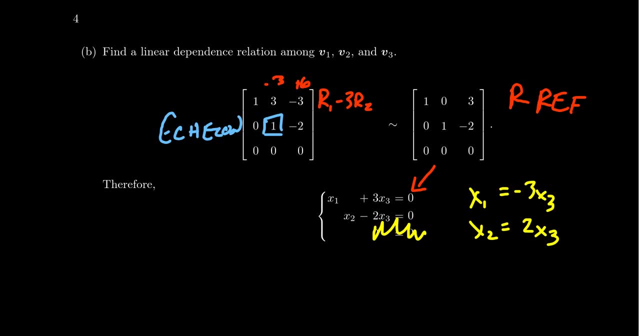 And we've then reproduced the trivial solution. What if we take x3, though to be something non-zero, Like if x3 is set equal to be 1, that means that x1 would be negative 3x3. And x2 is just 2.. And I claim that this, right here, is an example of a non-trivial solution. 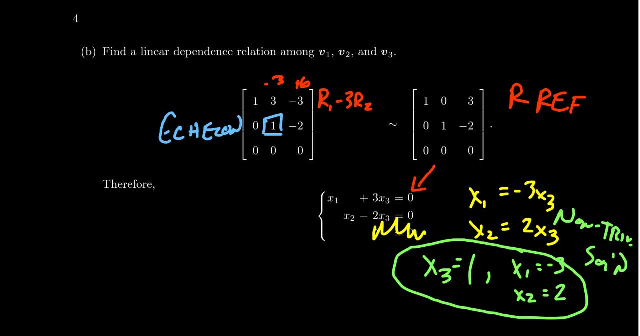 It's a non-trivial solution And this gives us a dependence relationship. We're going to take negative 3 times the first vector, which remember the first vector was the vector 1,, 2, 3.. We're going to take 2 times the second vector. 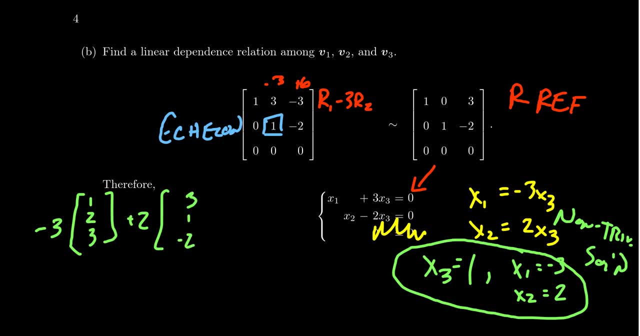 which you don't see on the screen here. but the second vector was 3, 1, negative 2.. And then we're going to take 1 times the third vector, which, recall that was negative 3,, 4, and 13.. 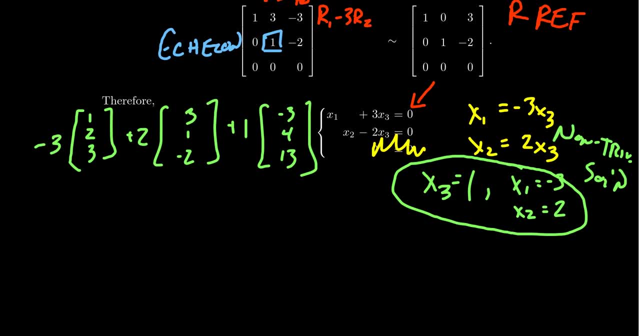 So what happens when we linearly combine these three vectors using these coefficients? You're going to end up with negative 3, negative 6, negative 9.. The second vector becomes 6,, 2, and negative 4.. The second one: you just times it by 1,. 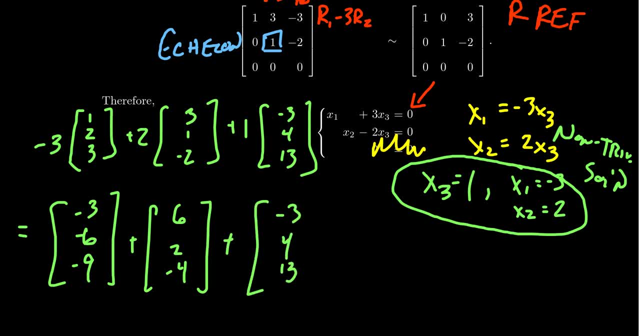 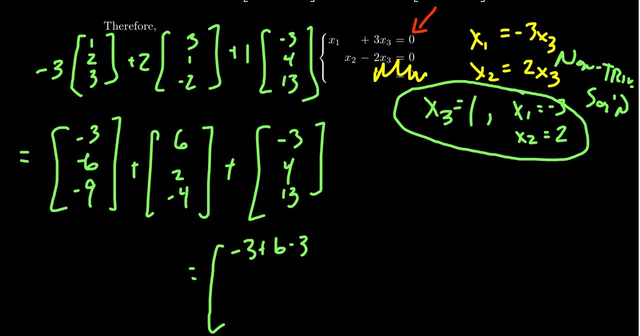 so you just get the same vector again: negative 3, 4, and 13.. And so, adding these together component-wise, you end up with negative 3 plus 6 minus 3, which, if I just stop you right there, that's a 0. 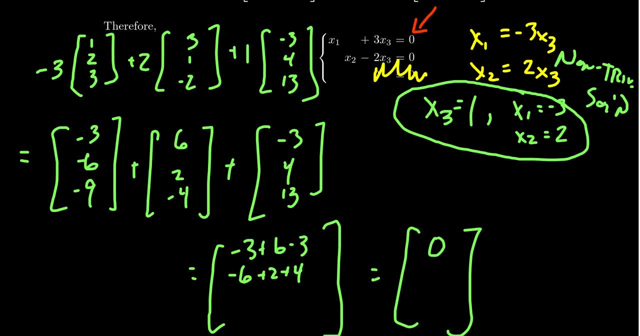 If we then take negative 6 plus 2 plus 4, that's also 0. And if we take negative 9 minus 4,, 9 and 4 give us 13.. Oh, looky there, 13. You're going to get 0 here. 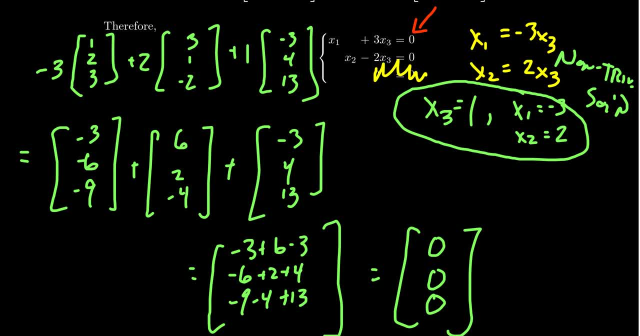 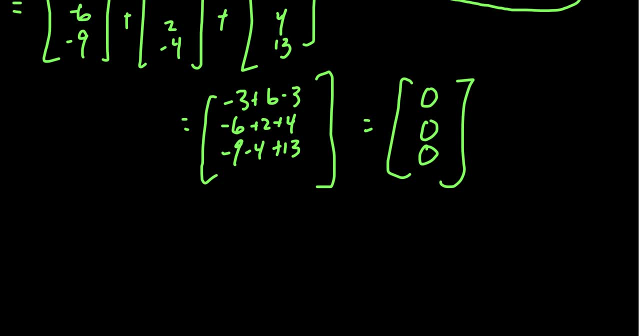 And so, in fact, this does give us a non-trivial way to combine the vectors together, And so what we now see here is we have this dependence relationship. We can see that negative 3, v1, plus 2 times v2,.